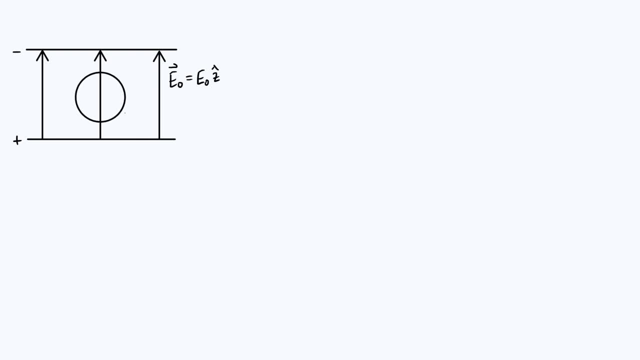 conducting sphere in. Well, let's draw that. let's put this sphere exactly at the midpoint of the two parallel plates. so conducting sphere now. it could be a hollow sphere, so just like a spherical shell, or it could be a completely solid kind of ball of metal. you would get the same result either way. Now let's think about intuitively. 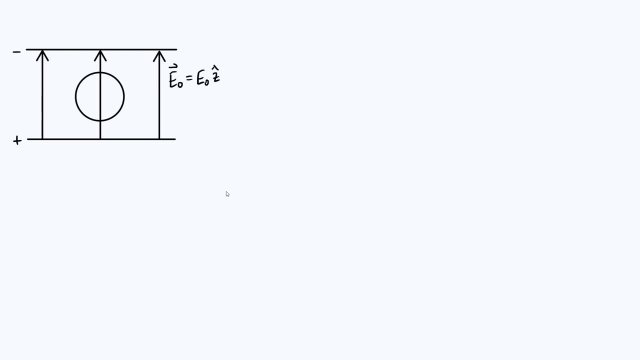 what we'd expect to happen. so, because the electrons in this conductor are free to move around, you would expect a build-up of negative charge near the bottom right, because the electrons are going to be attracted towards the positive plate and because, overall, the sphere has to be. 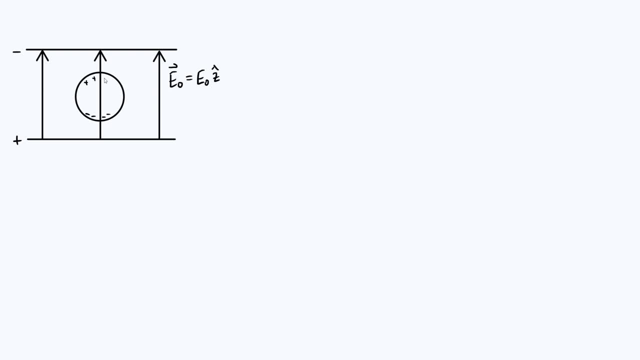 neutral, you would be left behind with an excess of positive charge on top of the sphere, like that. okay, and so you get this. intuitively, you would expect to get this charge separation, and that's kind of like a dipole right, because a dipole is just two oppositely. 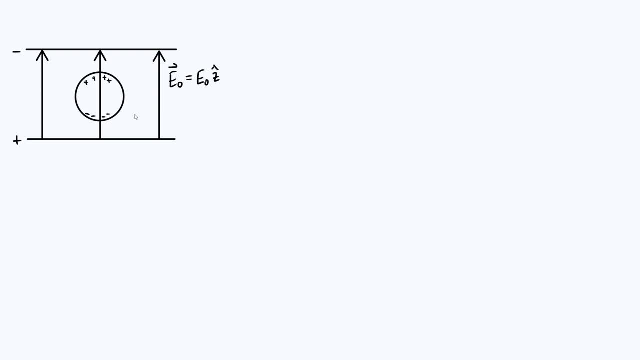 signed charges that have been slightly displaced from each other. Okay, so, based on that idea, what we're going to do is actually start this off not by thinking about a conducting sphere, but by thinking about a dipole, and then we're going to show that a dipole is actually equivalent to a. 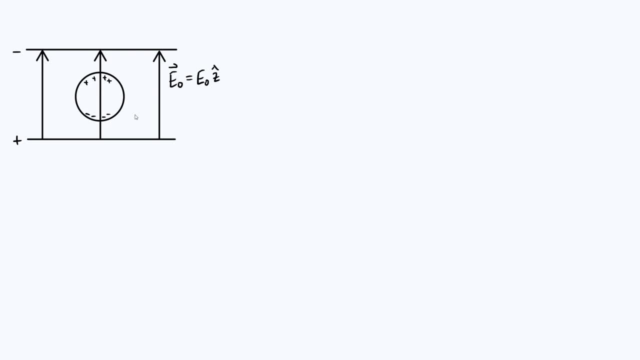 conducting sphere in this particular scenario. right, so what I'm going to do is say the origin of the coordinate system is going to be exactly in the center there, and let's consider what happens if we place a dipole moment defined by- sorry, a dipole whose dipole moment is given by a vector p, like that. if we 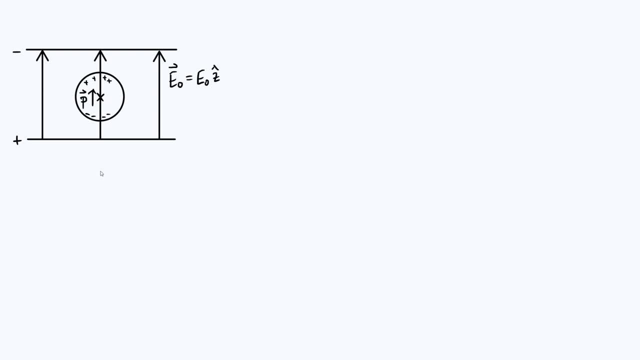 place that at the origin, in this uniform electric field. what is going to happen? so what we can do is use the principle of superposition to add together the potential associated with the dipole and the potential associated with the dipole and the potential associated with the dipole. 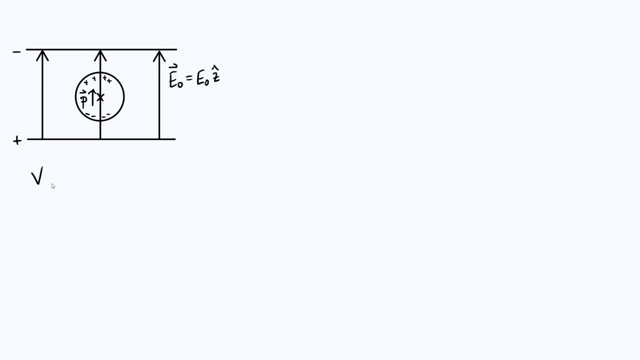 and the potential associated with the uniform field. right, so let's first write down the potential associated with a dipole. now, this is a standard result if you want to see where it comes from. I do have another video on that. but the potential of a dipole is p, cos, theta divided by 4, pi, epsilon. 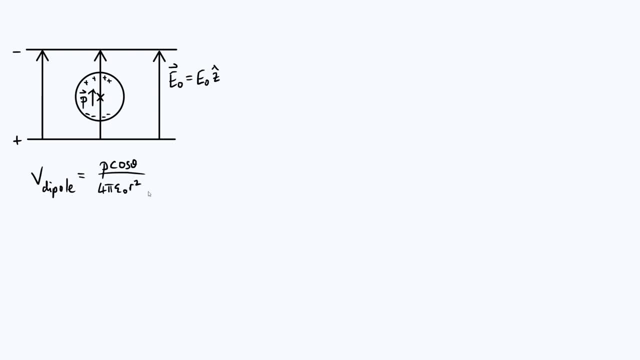 naught r squared, where p is the dipole moment and theta and r are just the standard spherical polar coordinates, right? what about the potential associated with the uniform field? that's just v subscript uniform. now we know that. well, this electric field e naught that is supposed to be given by minus the gradient of this potential, v uniform right. 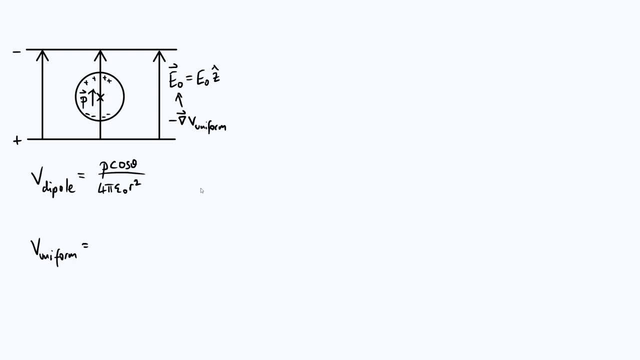 by definition of what the electric potential actually is, and so I guess by inspection of that, that fact, we can spot that the potential associated with the field is, has to be minus e-naught times the z-coordinate right. To convince yourself of that, just try taking the gradient. 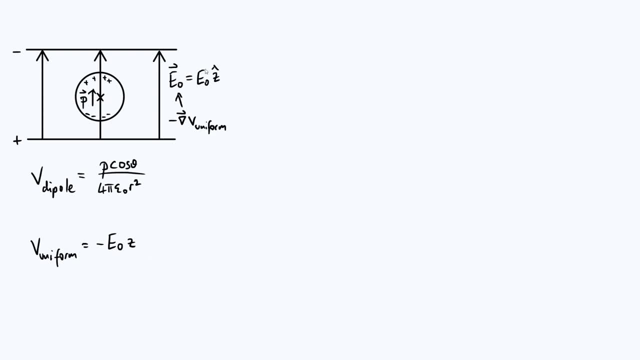 of that potential and you'll recover e-naught times the z-hat vector. Now, because the dipole potential is most naturally expressed in spherical polar coordinates, let's also transform this z into spherical polar coordinates. Now, this is a standard transformation. z is equal to r. 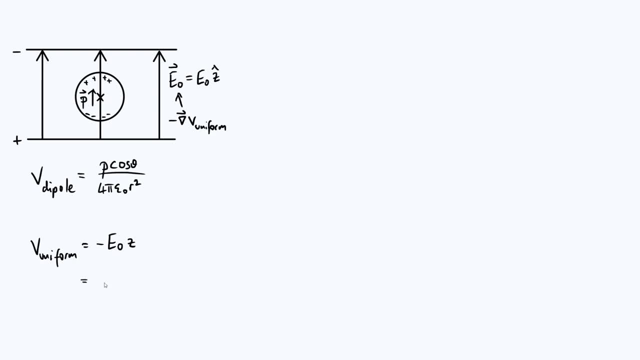 cos theta right If we're converting from cartesians to polars. So we can write that as minus e-naught times r cos theta right. So, by the principle of supervision, if we want to know what happens if we actually place this dipole in a uniform electric field, we can just add those. 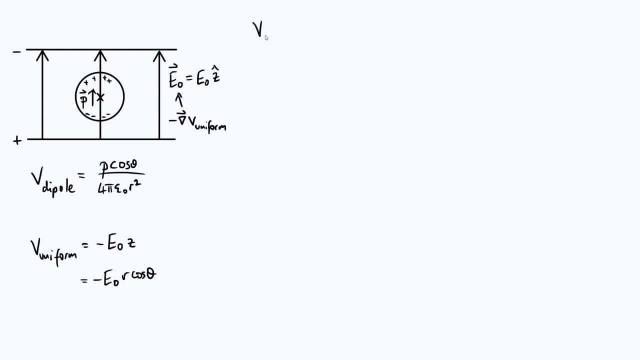 two contributions together, right. So we find that the total potential- let's call it v-tot- is just going to be p cos theta over 4 pi. epsilon-naught r squared, And we've got to subtract off this e-naught r cos theta. 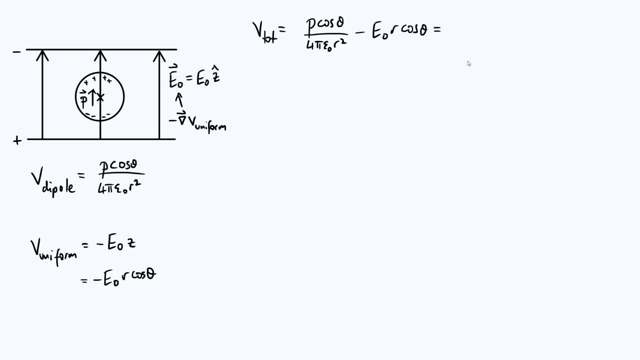 And what we can also do is factorize out a cos theta right. Both terms are proportional to that same angular term, cos theta. So we get p over 4 pi, epsilon-naught r squared minus e-naught r, all multiplied by cos theta. So the interesting thing about this is that the angular and radial 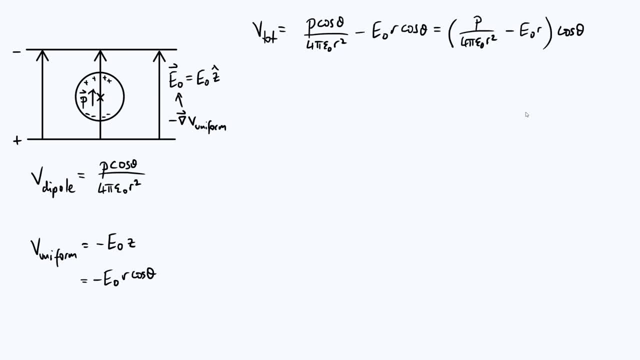 parts of the potential have kind of, they've completely decoupled from each other, right? So this bracketed term only depends on radius And this cos theta only depends on the angular part. well, the angular coordinate, sorry, theta. And so notice that there is a specific surface. 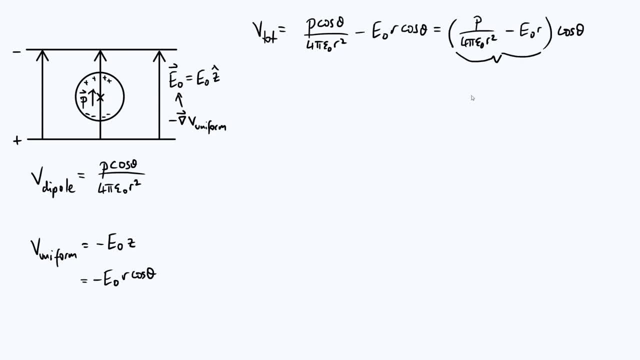 along which or over which, this bracketed term is zero And therefore the potential overall is zero. So let's think about the implications of that. right? We can say that the potential is zero if p over 4 pi, epsilon-naught r squared is equal to e-naught r. 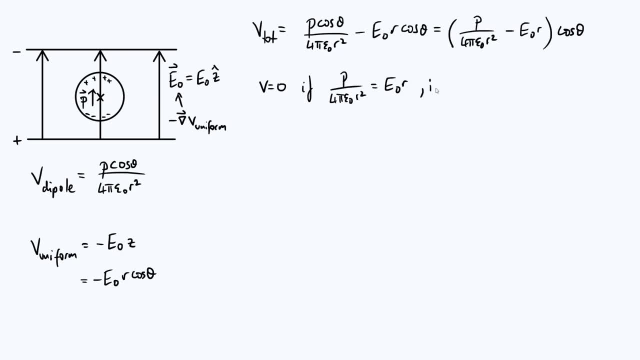 right, Because then the bracketed term is going to be zero, If we just rearrange that to make r the subject right. So multiply up by r, squared, divide by e-naught, and take the cube root. we find that this, the particular radius at which the potential is zero, is given by 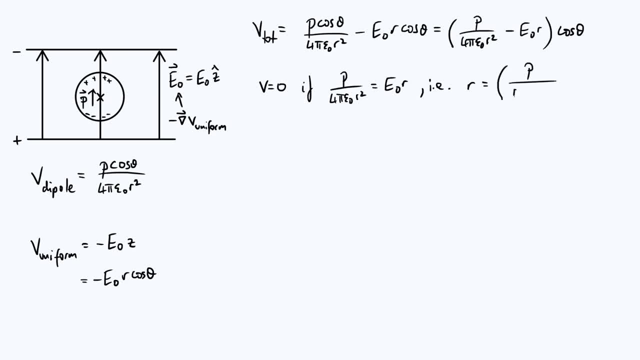 p over 4 pi, epsilon-naught, e-naught, all to the power of 1 third. And this defines a spherical surface right, Because it's just a surface of constant radius. So what we're saying is, if you put a dipole in a uniform electric field, there exists a particular spherical surface which is: 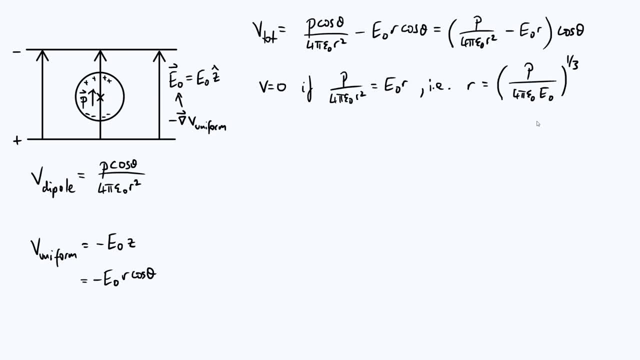 an equipotential surface right Because the potential takes the same value zero everywhere on that surface. So if you put a dipole in a uniform electric field, there exists a particular surface right Because the potential takes the same value zero everywhere on that surface. So 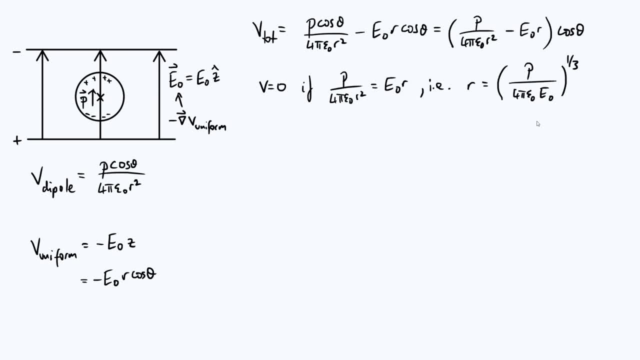 what we can do, then, is invoke the uniqueness theorem, which is another topic I have another video about, if you want to learn a bit more about that, where we're going to invoke the uniqueness theorem and say that, well, a conductor has to be an equipotential surface always. 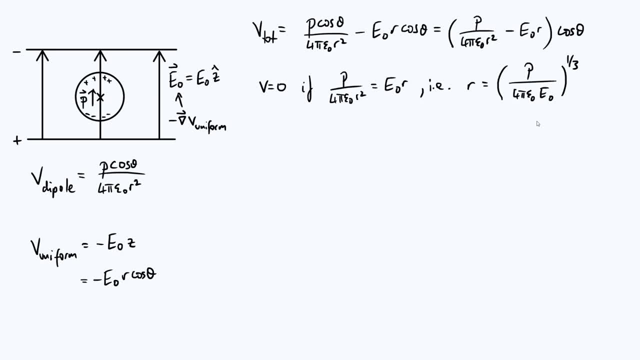 right? The idea with that is, if it wasn't an equipotential surface, then you would have this kind of constant motion of electrons along the surface, right? So this is the equation that we're going to use for the same function, right? So if it wasn't? 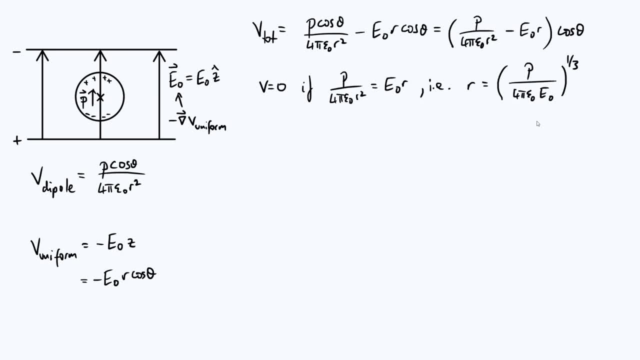 an equipotential surface, then you would have this kind of constant motion of electrons along the surface right. So the electrons would just move along the surface until they they kind of reach the distribution that ensures no further motion. okay, so the because the electrons are free to move in a conductor? 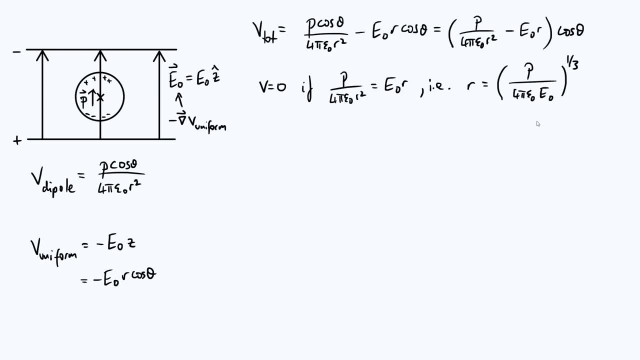 they always kind of redistribute themselves until they stop moving along the surface. so the surface of conductor is an equi-potential, which means we're actually free to place a conductor at this particular radius, spherical conductor at this particular radius, because that doesn't change the boundary conditions, because it's already an equi-potential surface, right, and so we have this. 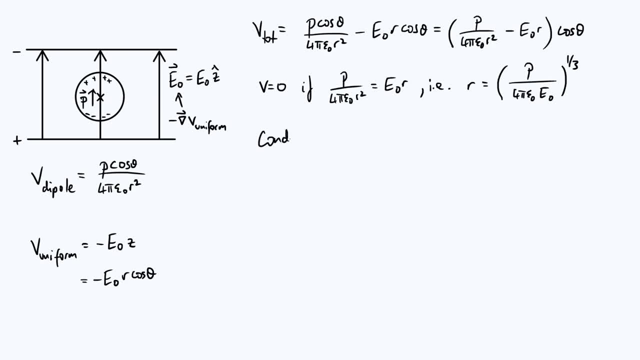 idea of an equivalence between, let's say, a conducting sphere. let's say the radius of this conducting sphere is going to be a. it's equivalent to, like the field you would get outside. that sphere is equivalent to what you would get by putting a, a dipole, at the center of the coordinate system, whose dipole moment is defined by that equation. 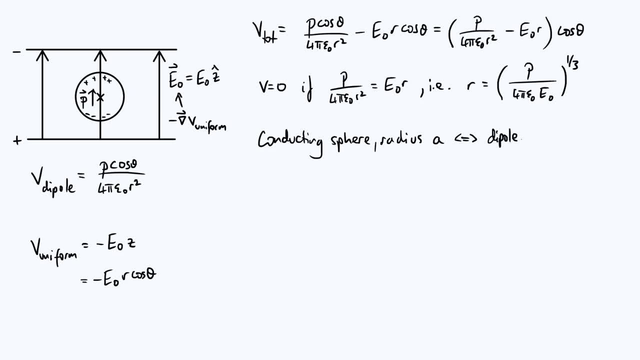 there, right? so this is equivalent to a dipole width, p equal to four pi. epsilon naught a cubed, e naught right, which has just come from rearranging that equation to make p the subject. okay, so we're just, we're appealing to the uniqueness theorem and saying that in either case you end up. 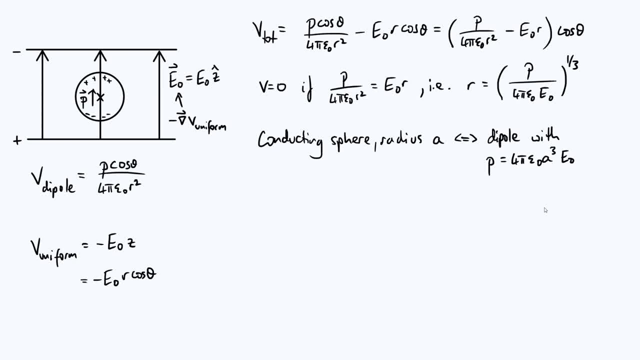 focusing there to be an equi-potential surface um at a at a particular radius, um, and so from the uniqueness theorem, the electric field outside that radius has to be the same in either case. okay, so one thing to notice about this is that the dipole moment that is equivalent to what you get with the. 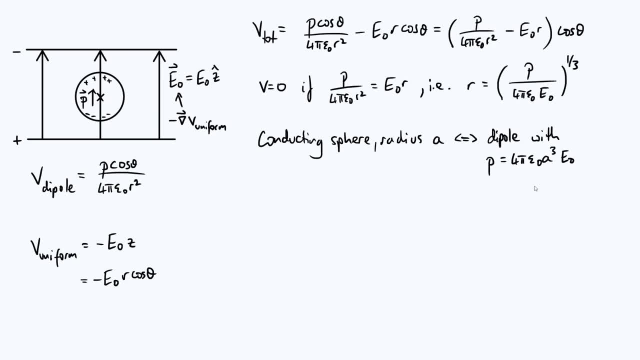 sphere is proportional to e. naught right. so if you make the um, the applied uniform electric field, bigger, the uh effective or induced dipole moment p just increases in proportion to that electric field. and we usually define um, all of that stuff, four, pi, Epsilon or a cubed to be a single coefficient which we call the. 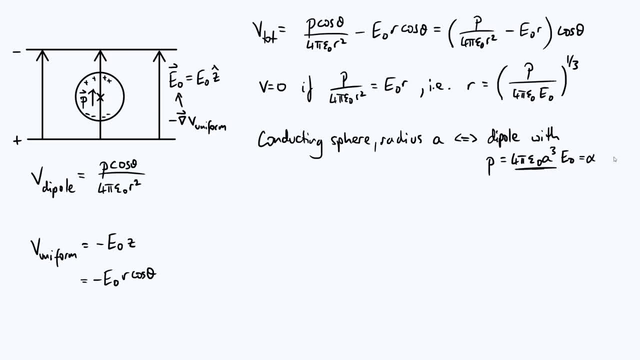 polarizability. okay, so usually written as Alpha, that's the same as Alpha, you know? um? okay, so what we can then do is go back to our expression at the top here for the total potential, and instead of writing this in terms of p, the dipole moment, we write it in terms of the radius of the equivalent conducting sphere. right? 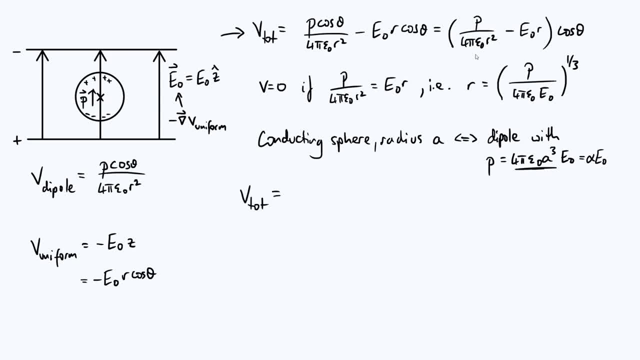 so what we get is the total potential is going to be: well, this first term in the brackets here, p over 4, pi, Epsilon or r squared um. we can rewrite that in terms of the radius a using that equation for the dipole moment, um, and that turns out to be the same as um. what's it going to be? it's going to be a. 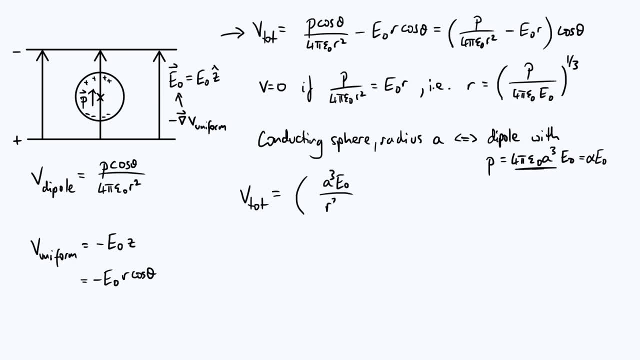 cubed, e naught over r squared, and the second term is still just um. e naught r right. so then we get this, this cos theta, which is still there, um. so we may as well also factor out an e naught right, so we can write that as a cubed over r squared minus r times, you know cos Theta? okay, uh, if we want the. 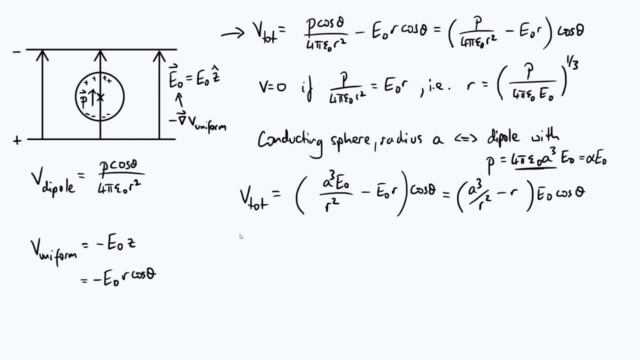 electric field, then we can just take the gradient of that and put a minus sign in front of it, and so the resulting electric field is going to be minus grad of v tot, um. in spherical polar coordinates, um. this gradient is going to be equal to minus dv by dr times. well, in the in the r hat. 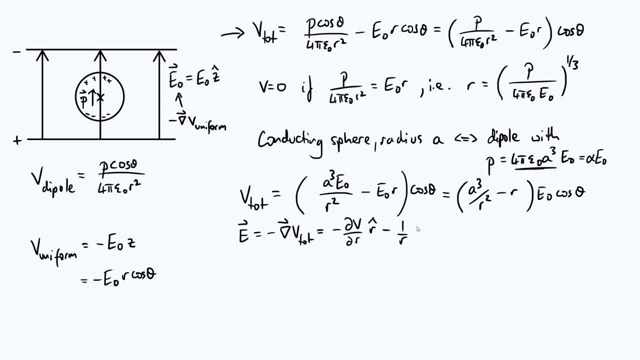 direction, and then the angular part is going to be 1 over r dv by d Theta in the Theta hat direction. okay, so if we go through do that differentiation to find um, the electric field vector, um, what do we get? well, the first part: we're differentiating with respect to r and so this a: 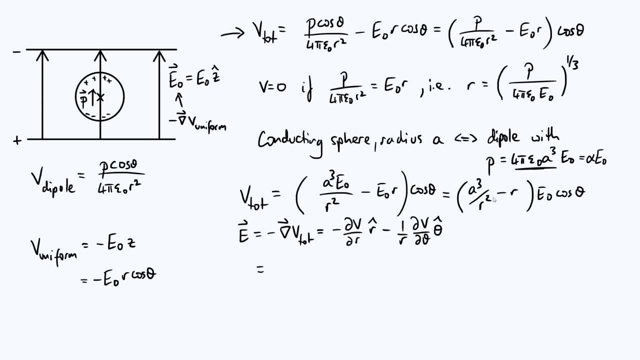 cubed over r squared is going to become a minus 2a cubed over r cubed. but then we've got this additional minus sign in the front right, so that ends up being just um 2a cubed over r cubed. second term becomes minus one. but again, uh, we, we've got an extra minus sign and so that's going to be a. 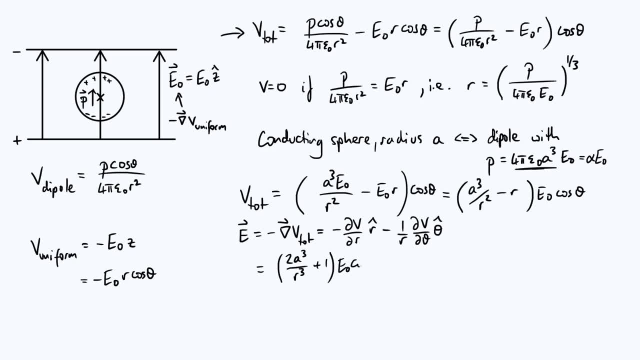 um, and then we've got our e naught cos Theta, and that's in the r hat direction, um, for this second term. well, the bracketed term stays as it is, but we divide the whole thing by r right, and so we add on: um a cubed over r cubed. uh, minus one this time. um, if we differentiate the angular part, we get minus. 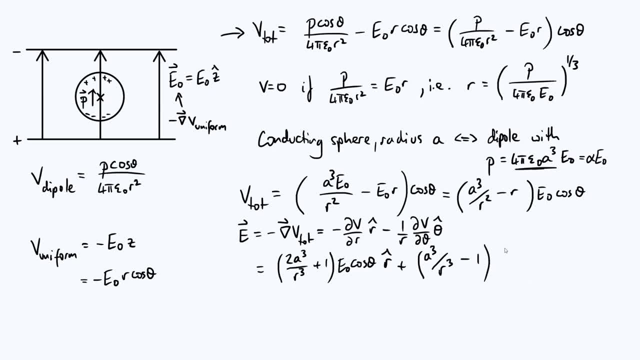 e naught sine Theta, but again there's a minus sign, and so overall we just get a positive: e naught sine Theta, like that, and that is in the Theta hat direction. so they, there you go. that's, that's our expression for the um, the overall electric field that you would get. 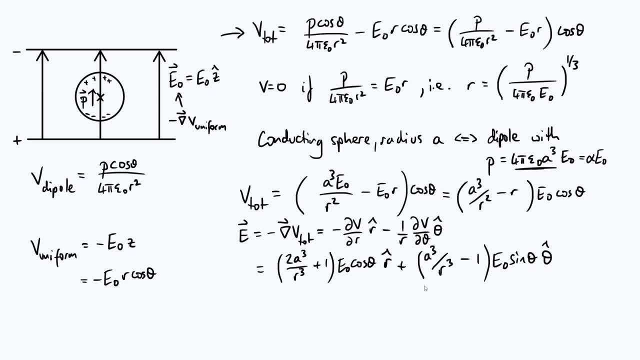 um, by putting this, this spherical conductor, into the uniform electric field. one other thing we can do is find the induced charge distribution and we're going to get that by considering the uh electric field just at the surface, um, like just exterior to the surface of the conductor. 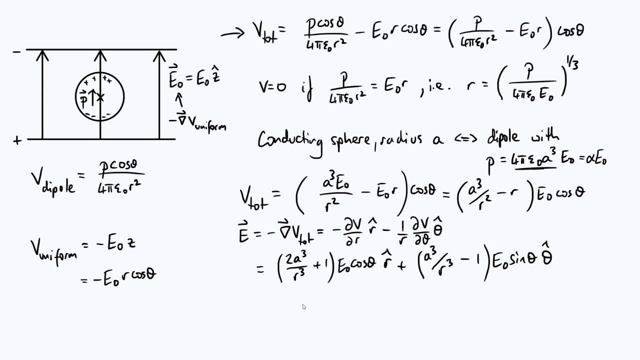 right. so if you go, if you're very close to the conductor, you can say the radius is roughly equal to a right. so r is is basically a and. so if we see what happens when we do that, if we set r equal to a, well this second term disappears, because a cubed over r cubed would be the same. 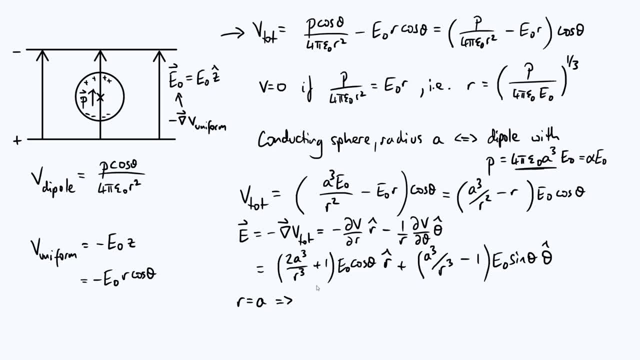 as one, and so that just goes to zero. um, the first term, uh, would become: we're going to get well again, a cubed over r cubed is one, so you've got two plus one in the brackets, which is three. so that would be e naught cos Theta times r hat. notice, by the way, that is purely radial, which it should be. 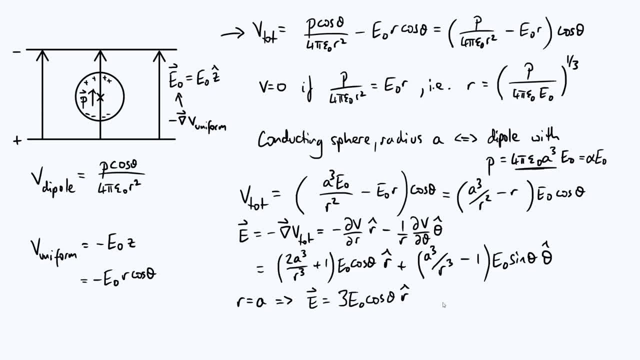 right, because an electric field in electrostatics always has to be perpendicular to the surface of a conductor, because the surface is an equipotential. so that's the electric field. now there's a way, a very simple way, to convert that into a charge distribution, which involves using Gauss's law and 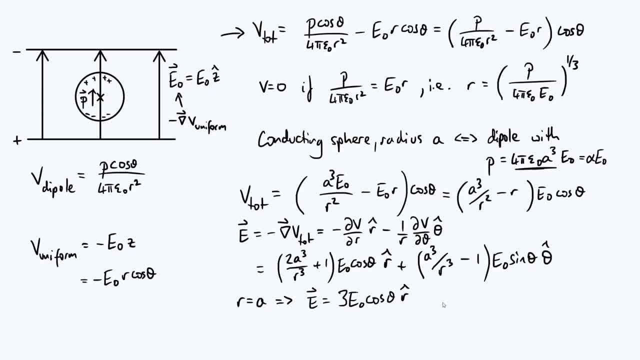 drawing a little imaginary box um around the the surface of the conductor and there's this general result that the electric field close to the surface of a conductor, um is given by just the charge density, surface charge, density, Sigma, uh, divided by Epsilon, like that. okay, if you haven't seen that and you want me to do a video on where that comes from, just 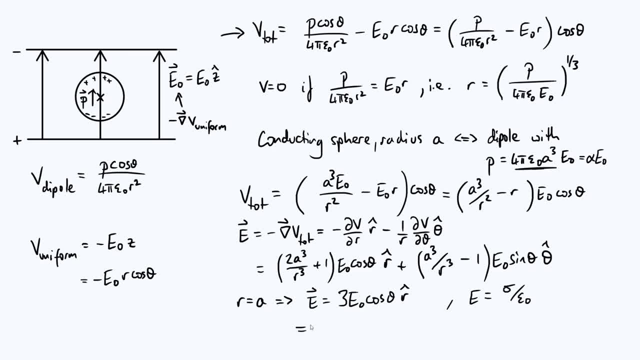 let me know in the comments. for now we're just gonna take that as a given and use that just to uh say that the surface charge density Sigma is just going to be three, Epsilon naught, E naught, um, cos, Theta. all right, so you get this charge density induced, which? 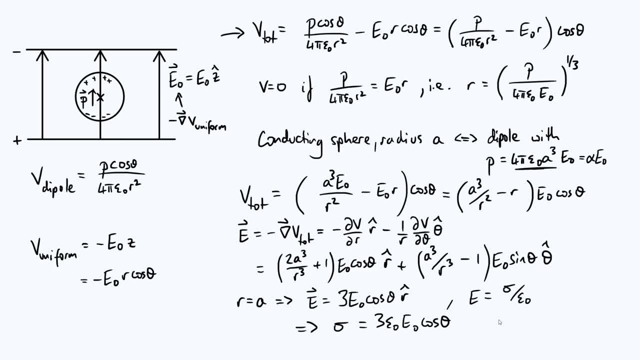 is proportional to cos Theta. all right, so there you go. one final point to note is: this only applies exterior to the um, to the, to the conducting surface inside the conductor, whether it's a or whether it's a solid ball of conducting material, the field is zero everywhere.